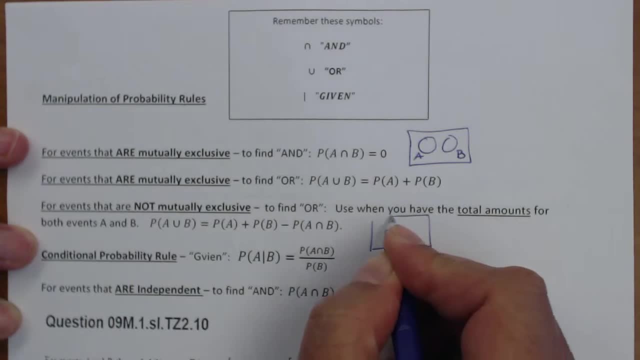 no overlap, But here for not mutually exclusive. what's going to happen is you're going to have the probability of A, which is this entire circle, and then you're going to have the probability of B, which is this one. So this overlap will be counted twice if we just added 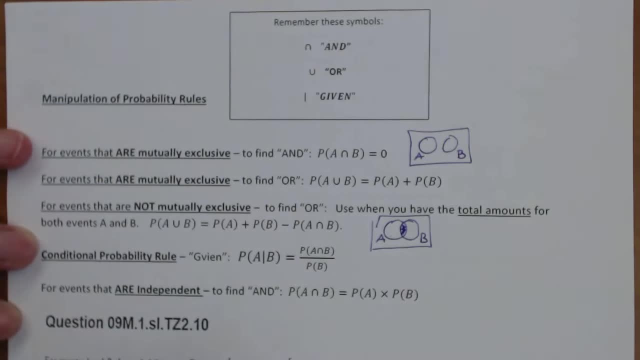 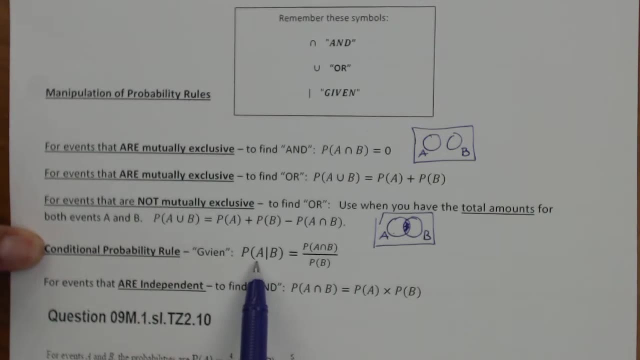 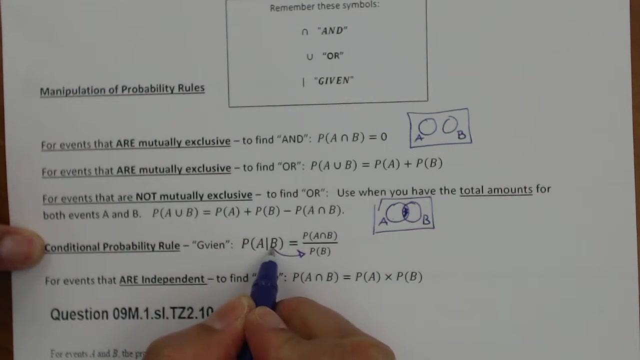 these two circles together. So we have to take out minus one of the middle parts that you added twice. So that's why that rule happens. Then you have conditional probability, where we have A given B, And so this denominator really relies on the given part. So we have 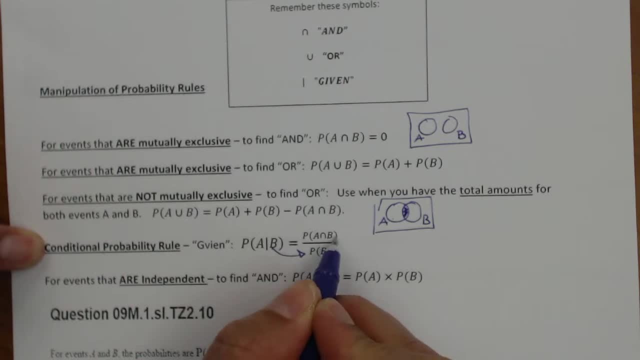 to find. the probability of B is the new denominator, And then the numerator is A and B happening at the set, both A and B, And then, lastly, we have independent events. So A and B. you can take the probability of A and multiply it by the probability of B for independent. 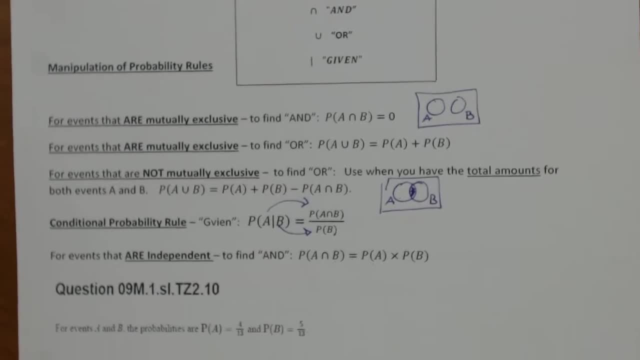 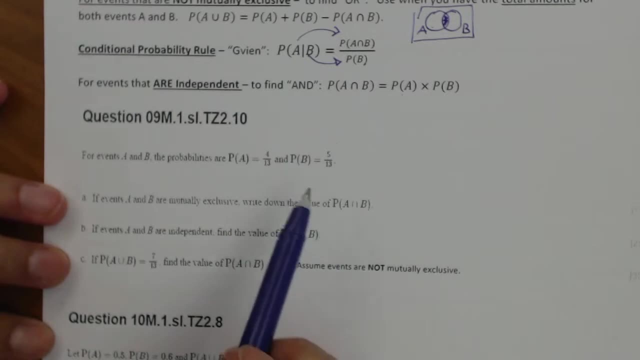 events. All right, so let's go through and utilize these rules and manipulate them. For this first question, here we have events A and B. the probabilities of A is four out of 13. And the probability of event B is five out of 13.. I'm sorry that if you can't see, 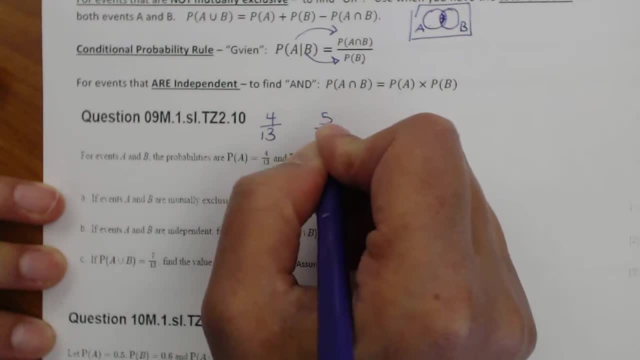 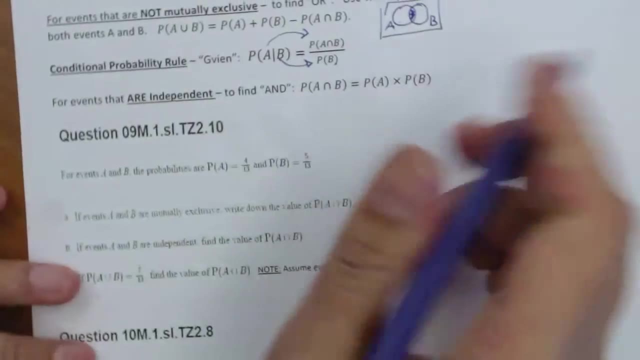 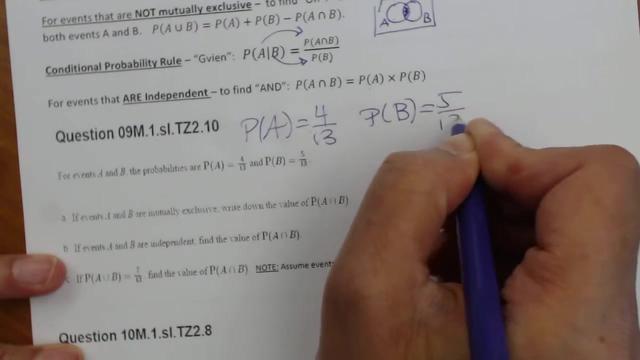 it here. I'll just rewrite it. It's very small on camera. So probability of B, that's not going to go right up here. probability of A is going to be four out of 13.. Probability of B is going to be five out of 13.. So that's what these, these say. So that's what these. 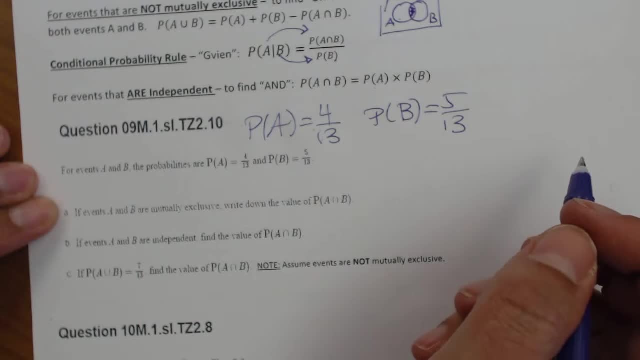 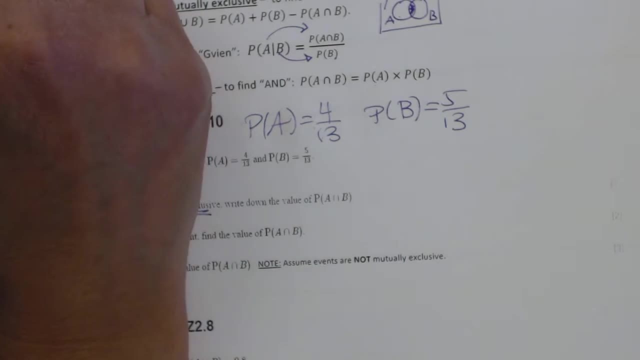 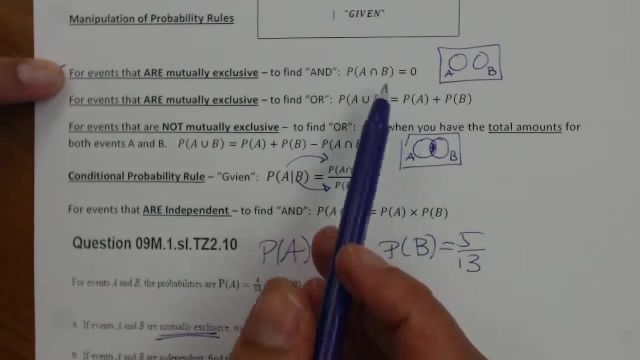 say: right here, All right. So part A: if events A and B are mutually exclusive, we have to write down the probability of A and B. So the key words here are mutually exclusive. So if you look up at the mutually exclusive, just start it right here. Rule we see to find. 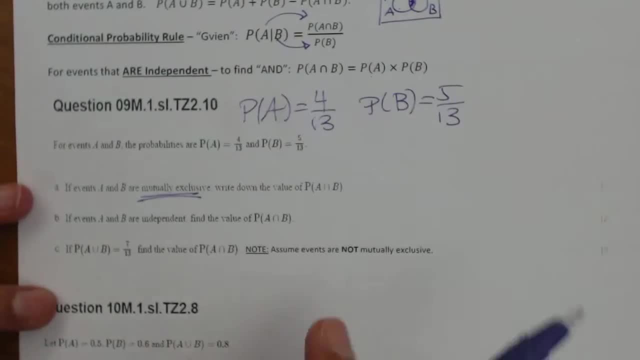 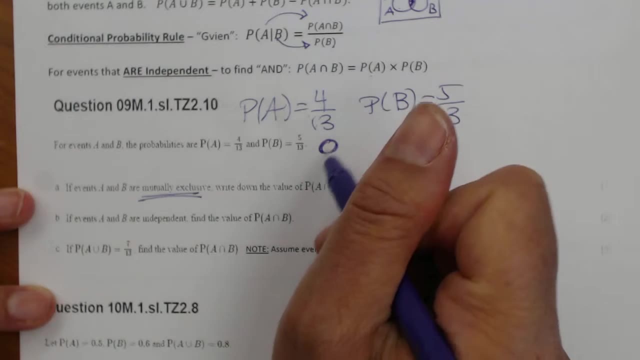 the probability of A and B? it will. it can't happen. So the probability is going to be zero. So the answer to this question is going to be zero. So that's what you would write down. Please do not put the slash through it, because 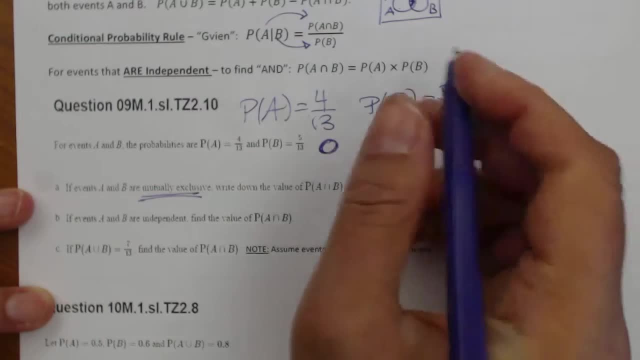 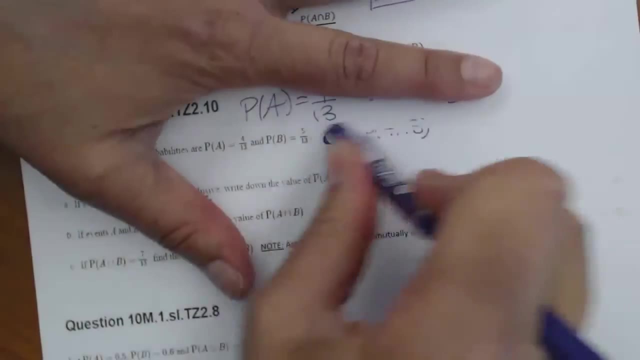 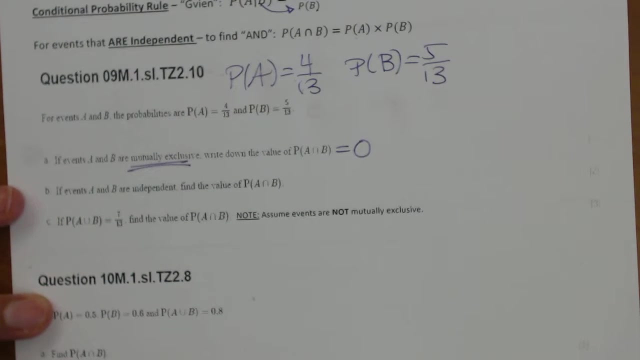 that means empty set. That just really just write the number zero. So zero equals the probability of A and B, And that's all because. and that's all because they are mutually exclusive. Get tired, some, writing it down. So this equals zero. There you go. Okay, the next one. if events A and 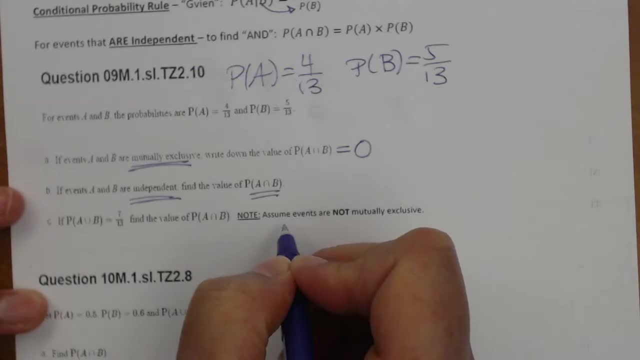 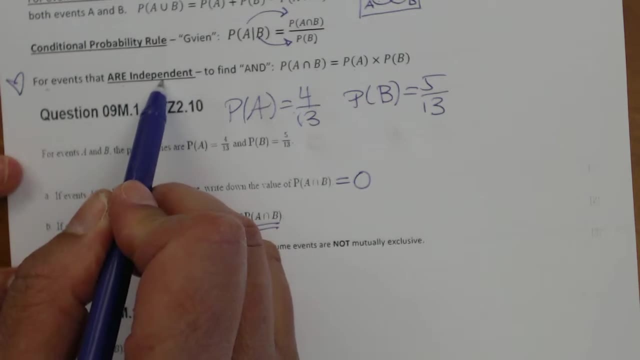 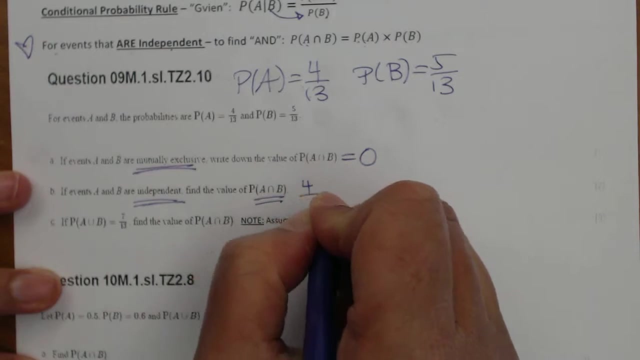 B are independent, find the probability of A and B. So what we have to do is: let's look at our independent rule. So we're right here For events that are independent- probability of A and B. We multiply them together, So we have those two probabilities. So let's multiply them. 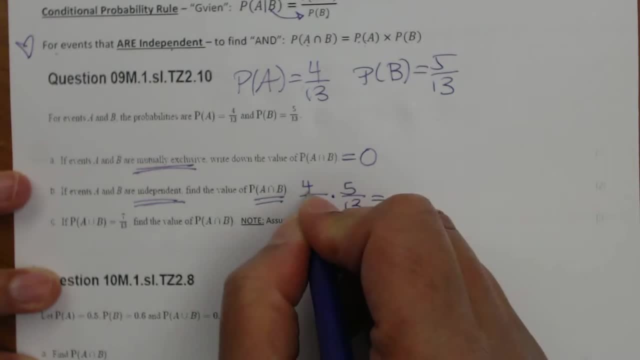 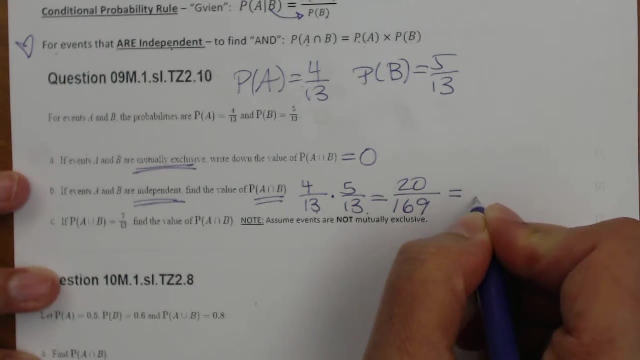 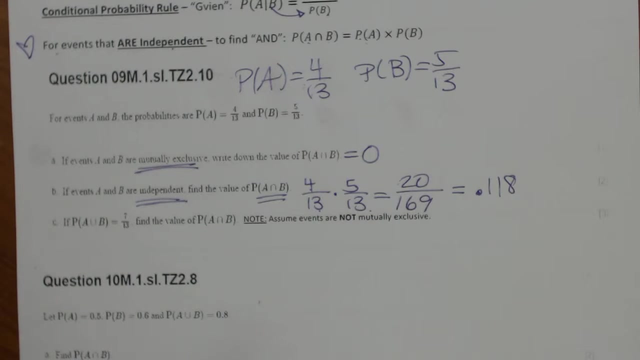 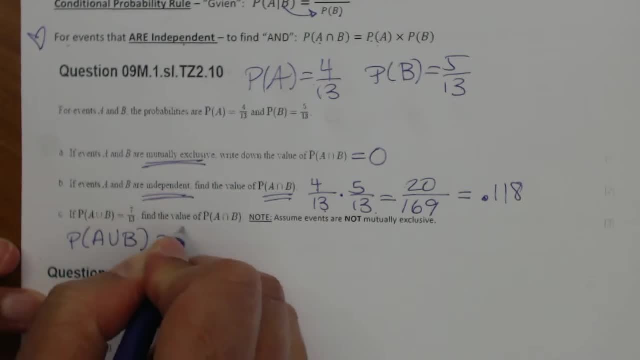 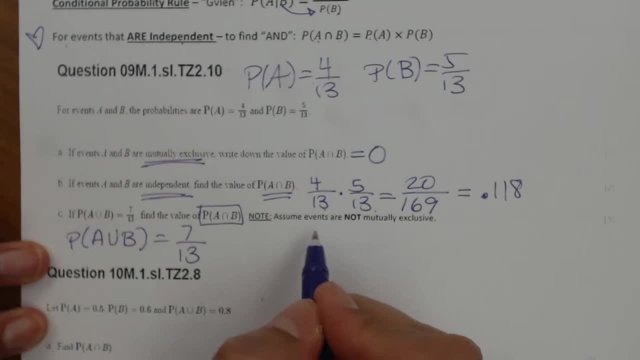 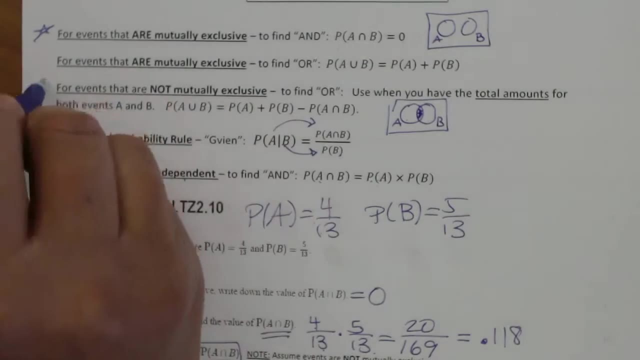 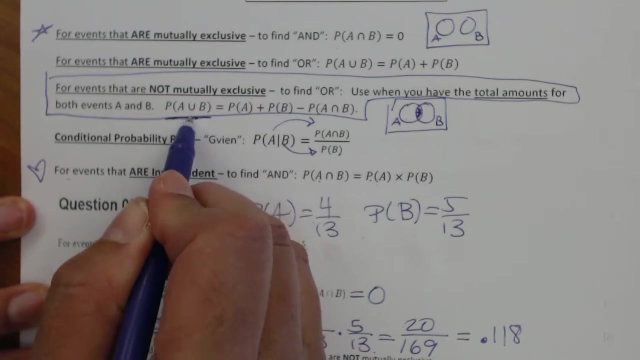 seven over 13.. I just rewrote it for you. Find the value of A and B? No, assume events are not mutually exclusive. So, because these events are not mutually exclusive, we're going to be using this rule right here. So they gave us the probability of A or B. They gave 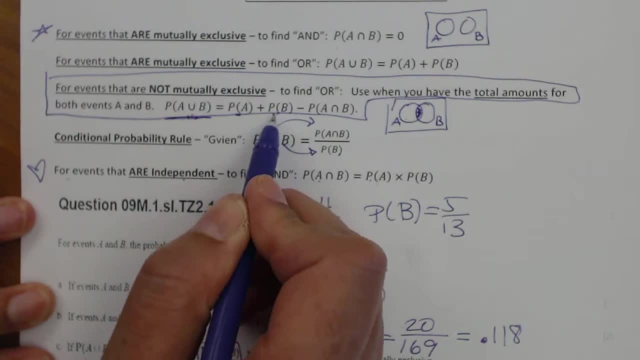 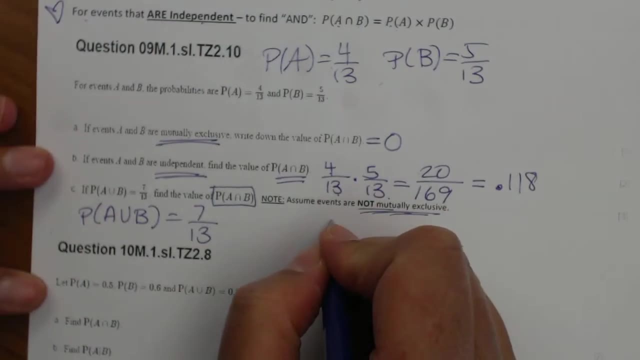 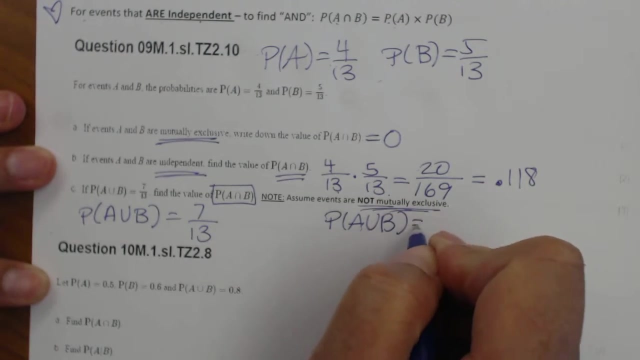 us this: They gave us the probability of A, They gave us the probability of B, So now we just have to find the missing a and b probability. So the rule that you're going to be using- and I'm going to do this out- probability of a or the probability of b equals the probability. 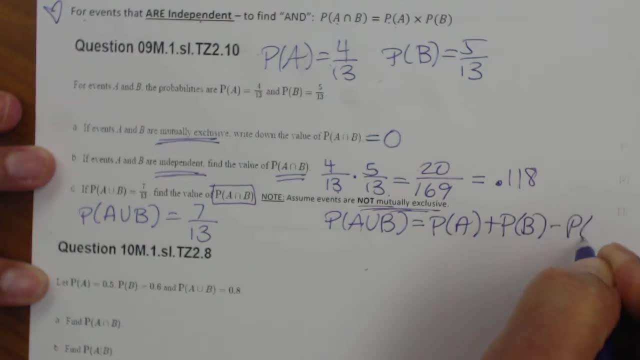 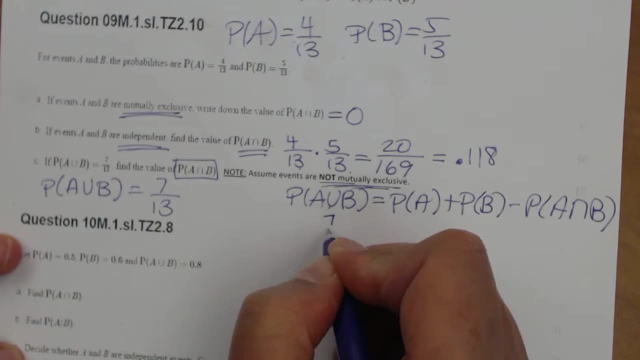 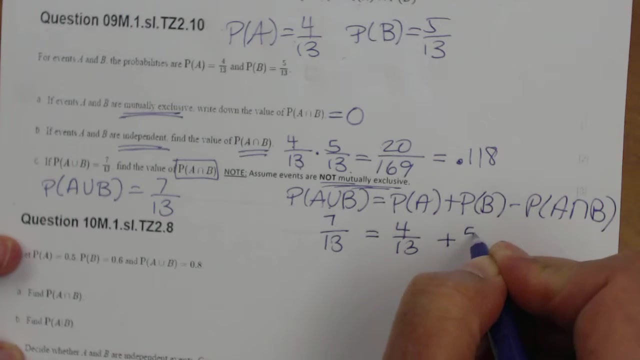 of a plus the probability of b, minus the probability of a and b. So let's just fill in what they gave us. the probability of a or b is seven out of 13.. The probability of a is four out of 13.. The probability of b is five out of 13 minus this is a minus and that's what's. 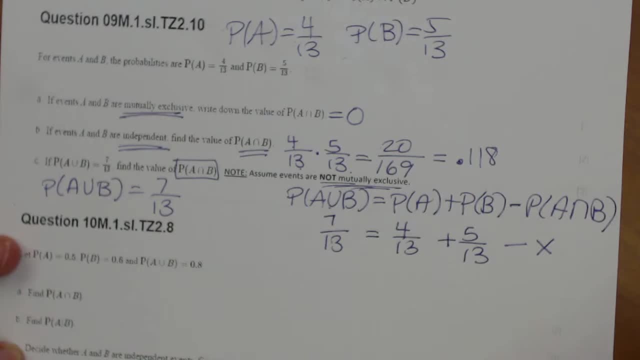 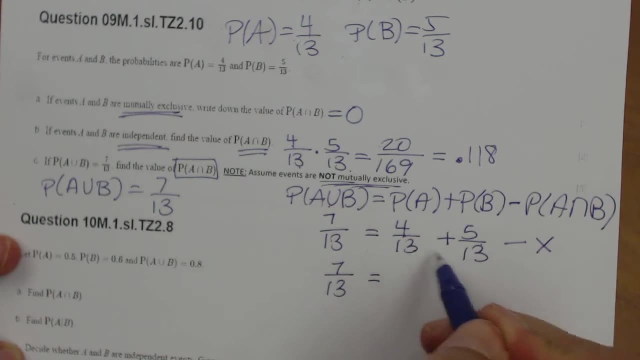 missing. So I'm going to just make that x, because that's what they want you to find. So now you can simply change this into decimals If you want. I am going to do the fraction just to show you some fractional work Here. these have the same denominator, so we can. 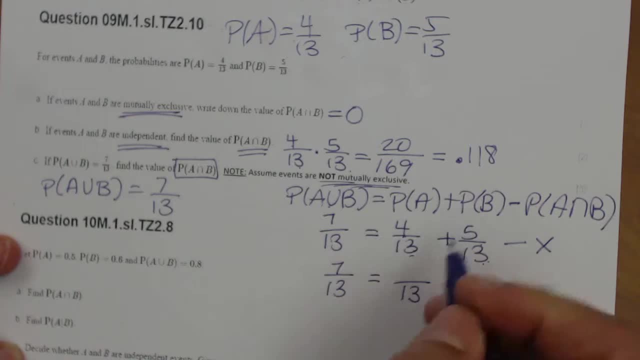 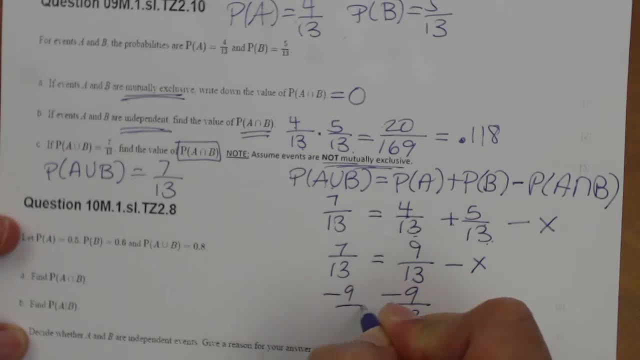 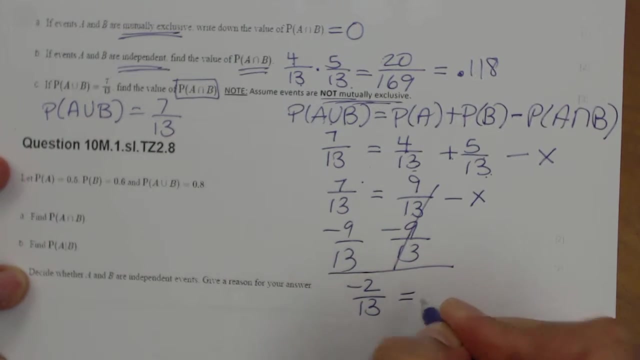 add them. we keep the denominator. that's why we need the same denominator and we add the numerator. So that's nine minus x. we need to solve for x, So we're going to subtract nine 13.. From both sides that cancels out seven, 13 minus nine 13.. Again, keep that common denominator. 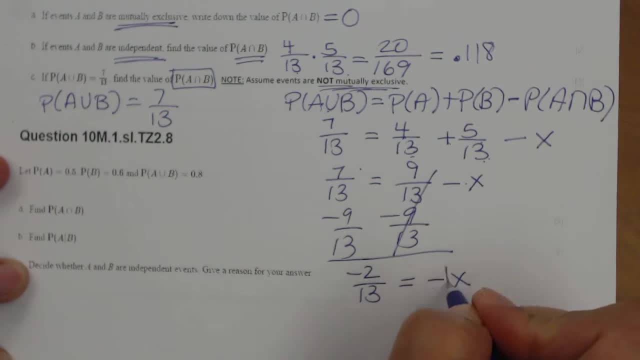 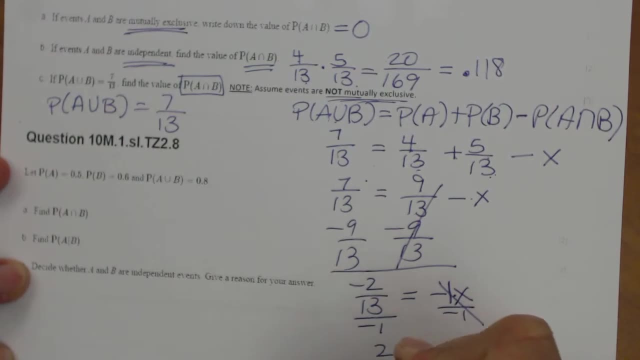 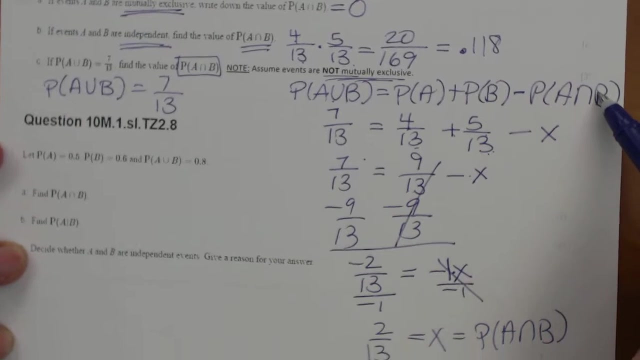 equals two, 13. And that is equals negative x. So this is really a negative one in front. So I'm going to divide both sides by negative one. So x is going to be two, 13. And that does equal the probability of a and b. So what we did is we use this rule. we use this. 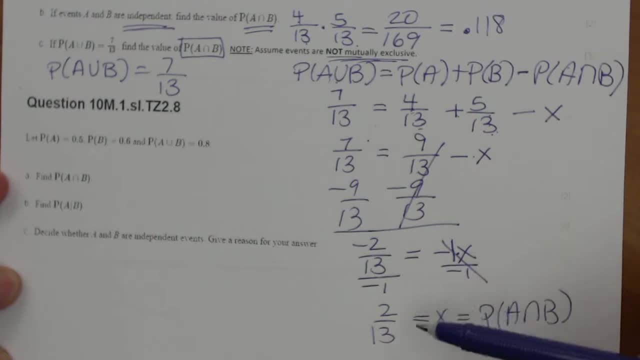 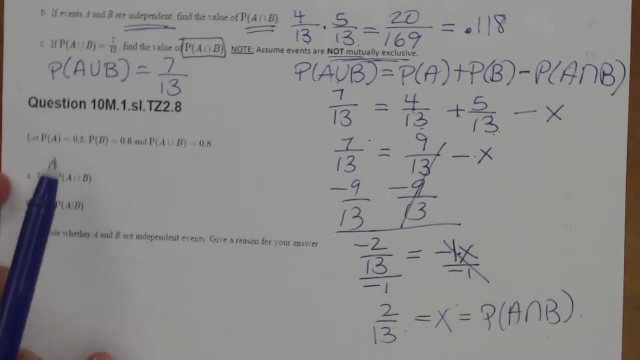 rule. we substituted our information in And we actually solved for the probability of a and b, which is going to be two, 13.. Okay, the second one. let the probability of a be point five. the probability of BP, point six. 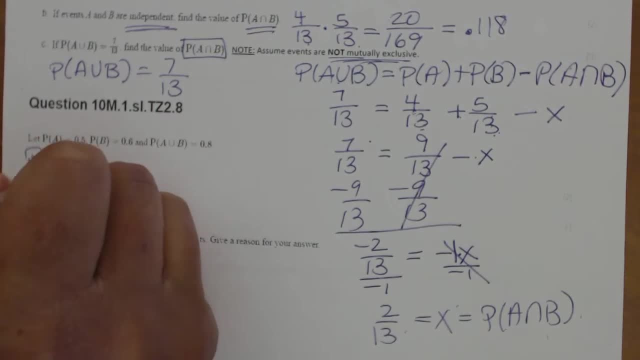 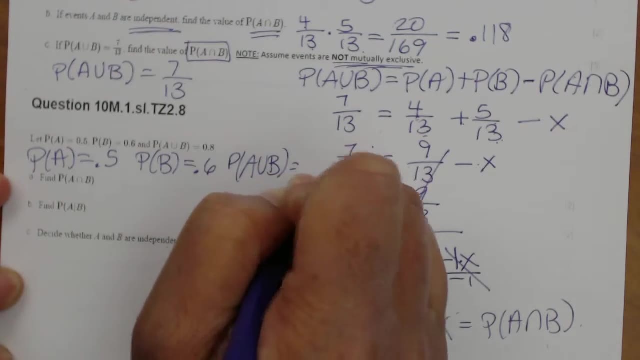 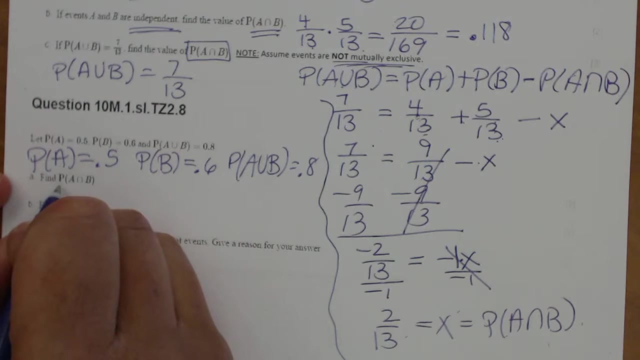 and a or B is point eight. So I'll rewrite it: probability of A is point five, probability of B is point six, probability of A or B is point eight, And then I'm just going to put a little line right here, Okay, So let's go through and see what they want to find Here. 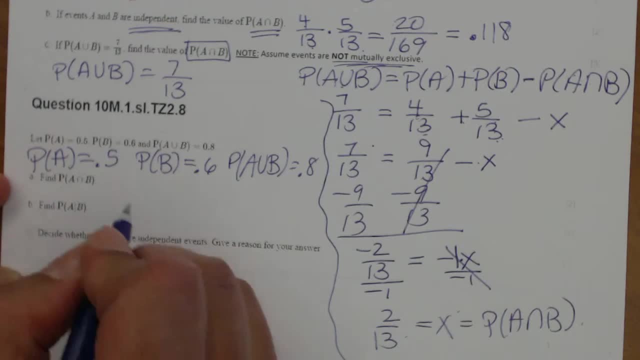 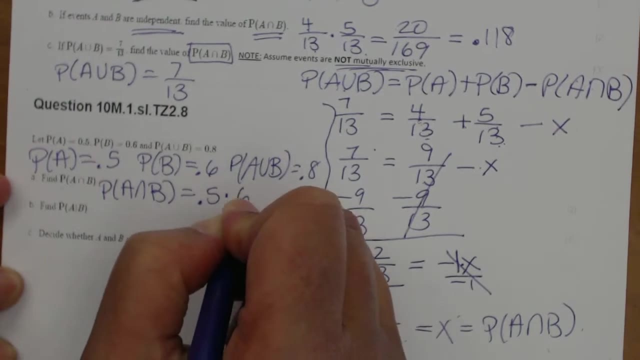 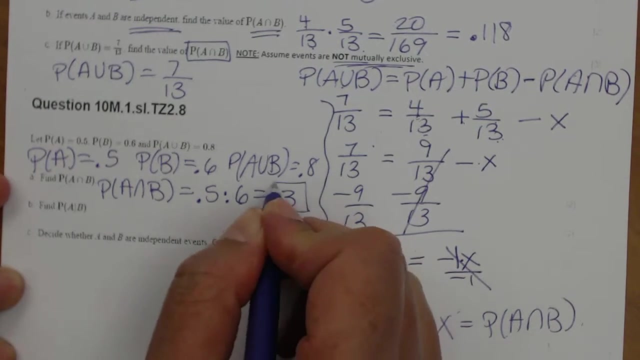 it says says: find the probability of A and B. So probability of A and B, let's use the independent rule: probability of A and B equals the probability of A times the probability of B. So point five times point six is point three. So that's that answer. Part B: find. 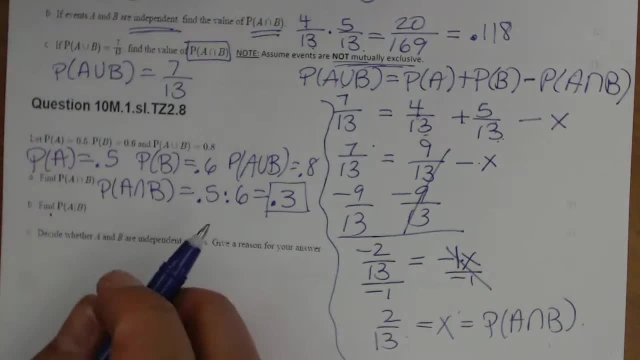 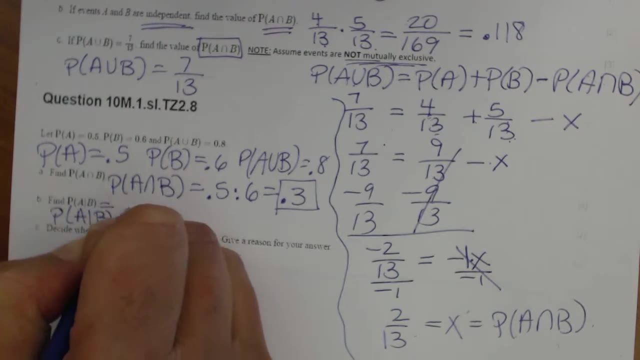 the probability of a given B. So what we have to look for- and I'm going to do this here- probability of a given B. So now the denominator is going to be the probability of B. that's my denominator. So let's look, denominator point six. So remember, what's given is now our new denominator, our. 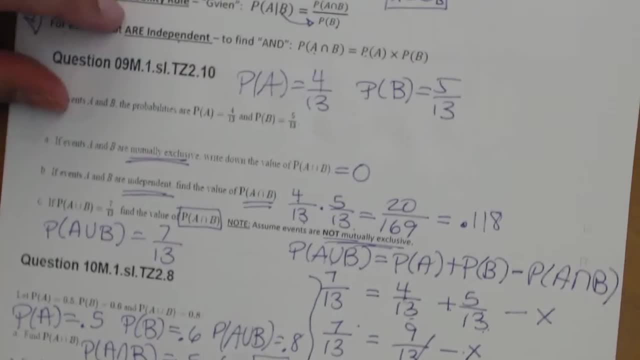 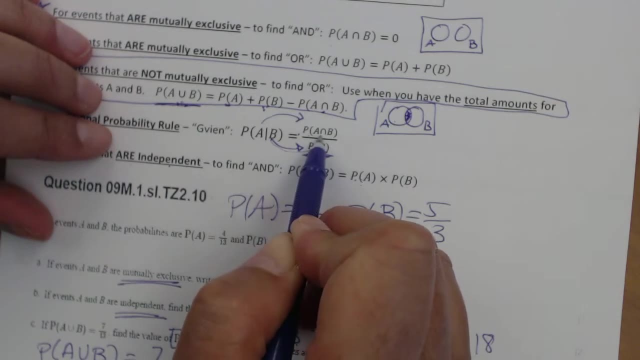 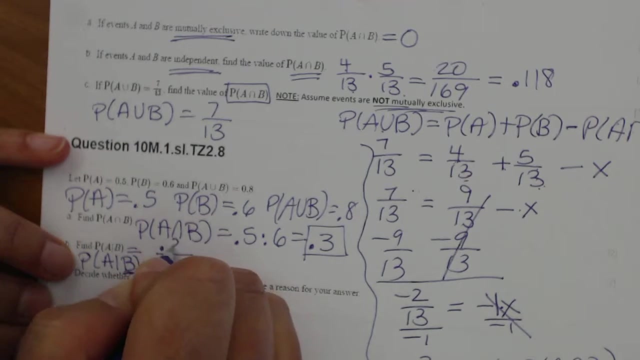 numerator is going to have to be. and if we look up here, here's our denominator, that's B, our numerator is the probability of A and B, And so I think I just recall that I found that, I found that here A and B is point three, So that's the numerator, So we have point. 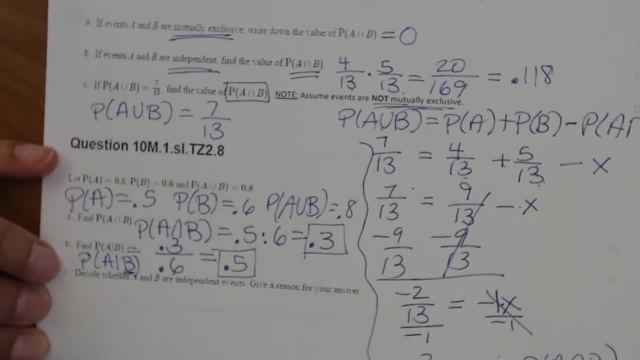 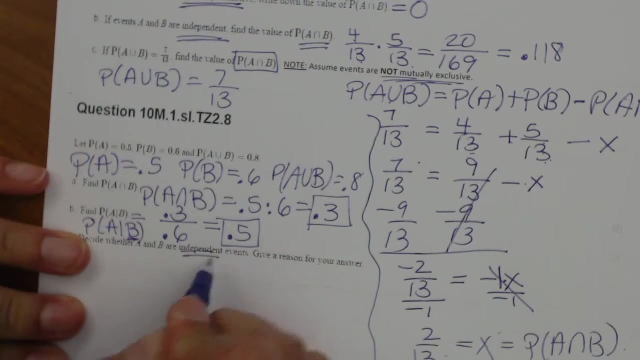 three divided by point six, and that comes out to be point five, And so that's our probability of A given B. it's just A and B, which is this. we've just found it divided by B, which was this year. they gave that to us, Alright. part C decide whether A and B are independent. 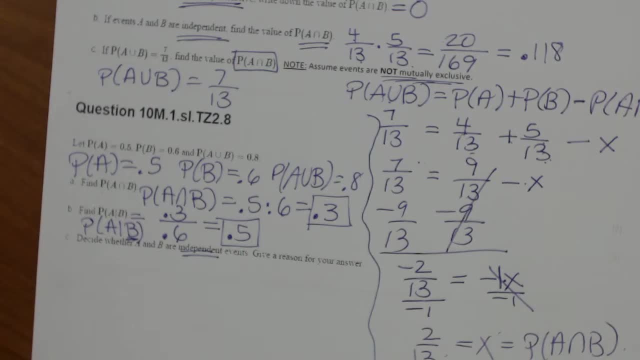 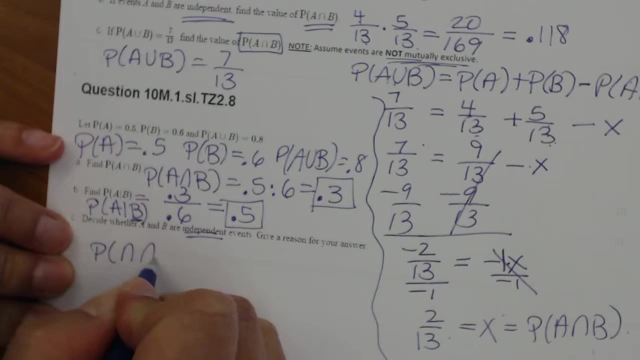 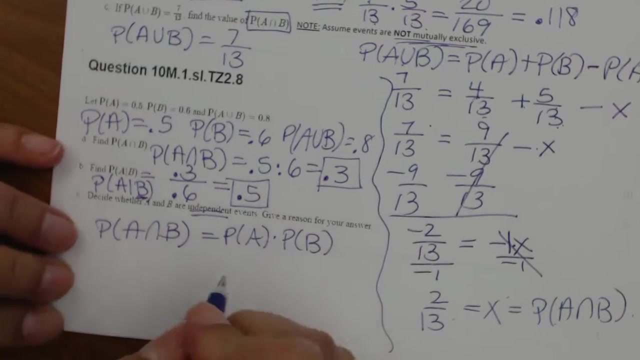 events give a reason for your answer. So this is what we're going to do. So if they're independent events, then that means that the probability of A and the probability of B equals the probability of A times the probability of B. So probability of A and B, point three: 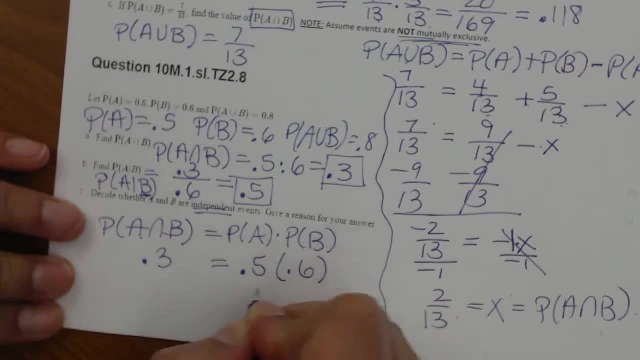 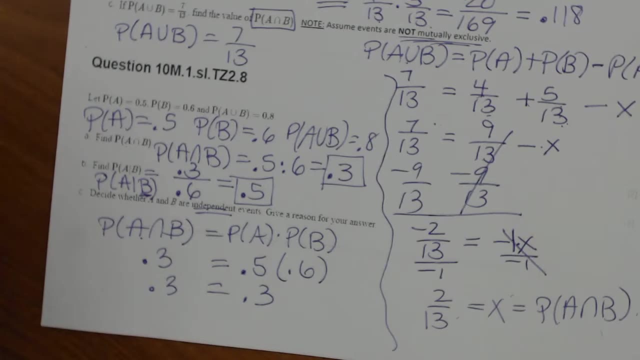 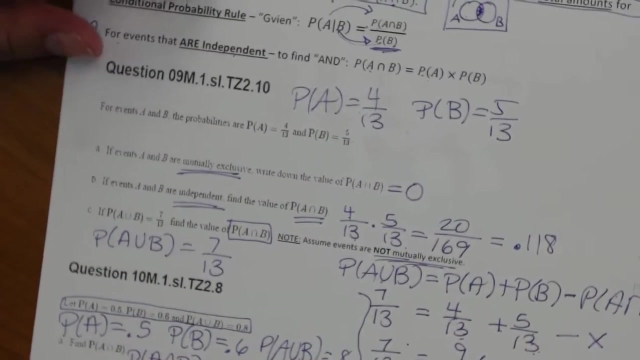 we got that by multiplying point five times point six, which point three equals point three. However, let's also see if we can prove it using the OR rule. So we have this information. So what I'm going to do is I'm actually going to write this down. I'm going to write this. 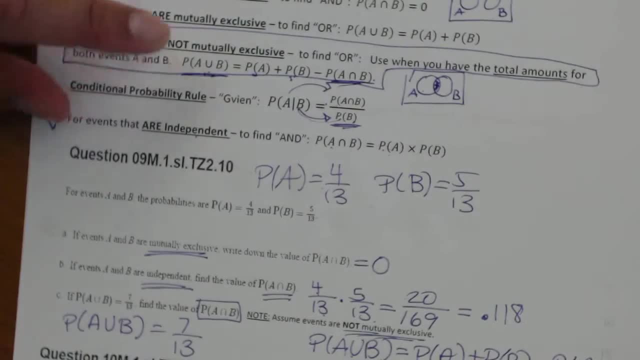 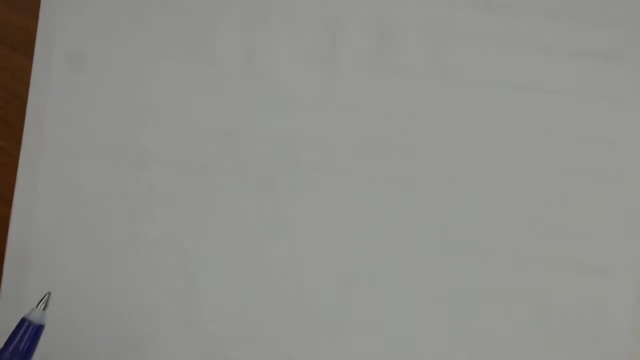 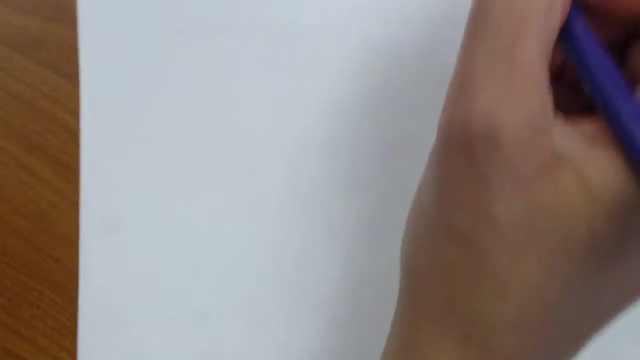 rule down and I'm going to see if this also comes out to be point three, And I'm actually I'm going to do that on the back of my paper, So I'm going to transfer this information. So it said: the probability of A is point five, the probability of B is point six and the 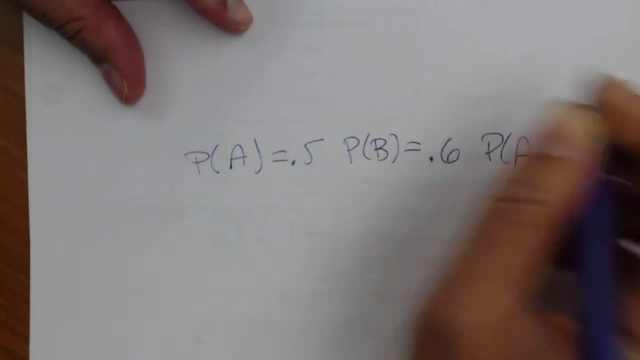 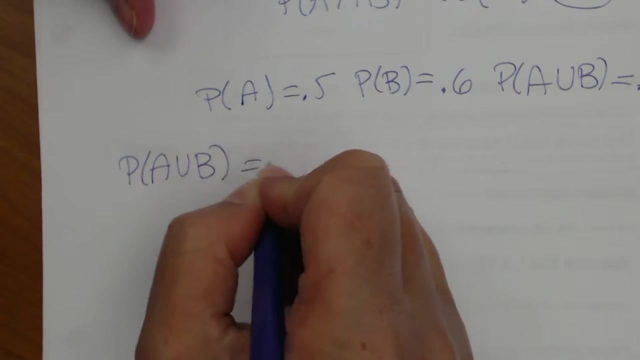 probability of A or B is point eight. Now I found the probability of A and B. if they are independent, it would be point five times point six, which is point three. Okay, so this is what we're looking to get, So I'm going to be using. probability of A or B equals the. 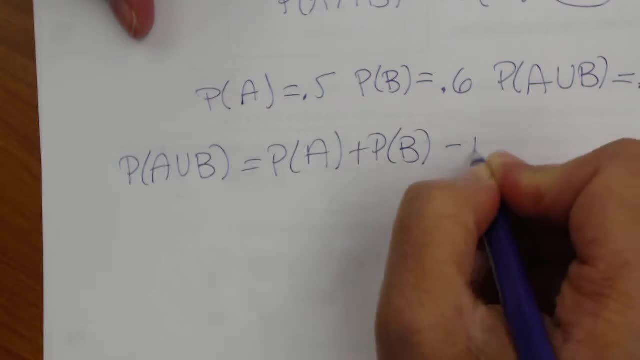 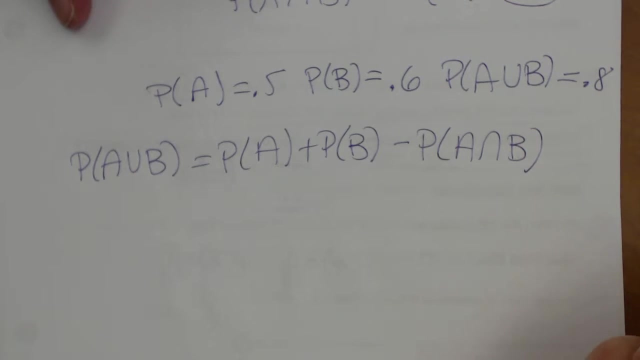 probability of A plus the probability of B, minus the probability of A and B. So let's substitute these numbers in and see if I get point three using this one. So I'm just manipulating these formulas to see if everything works. So A or B, so that's point eight, equals the: 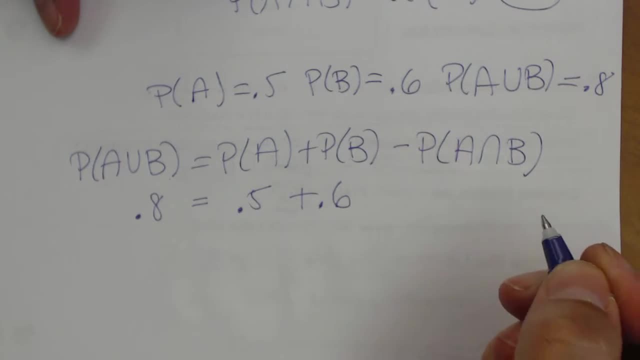 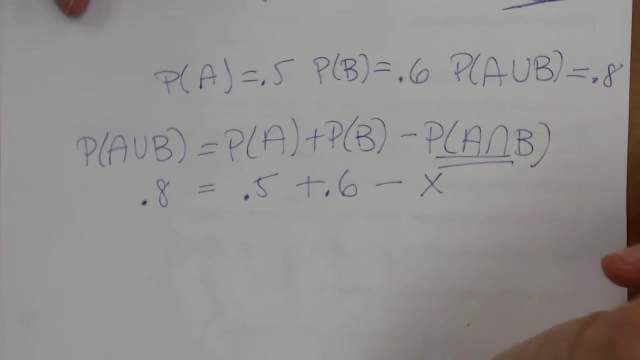 probability of A, which is point five, plus the probability of B, Which is point six minus. I don't know what this is. I'm looking for this to be equal to this if they are independent. So let's see what happens. So point eight equals point.